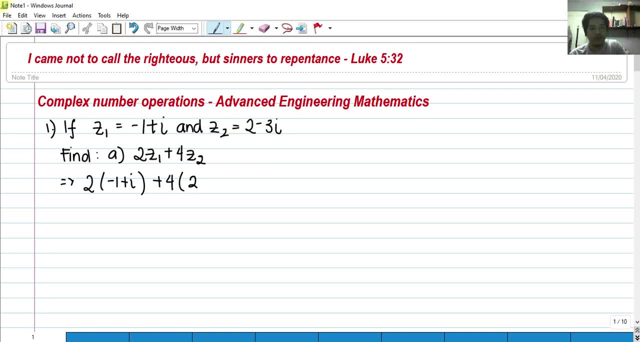 Then we're going to apply the basic operations such as the distributive, the associative, the properties in basic algebra. Then we have plus 4 times the z sub 2, which is 2 minus 3i. So simply evaluate: 2 times negative 1 is negative 2.. 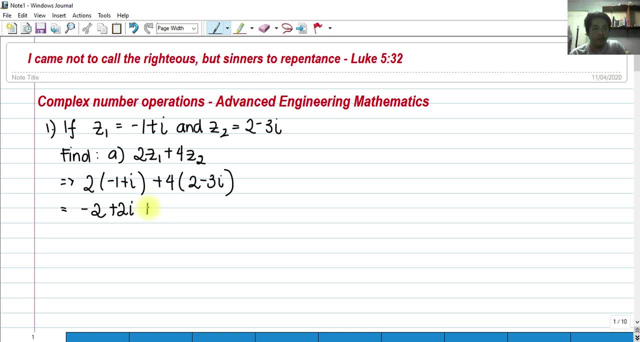 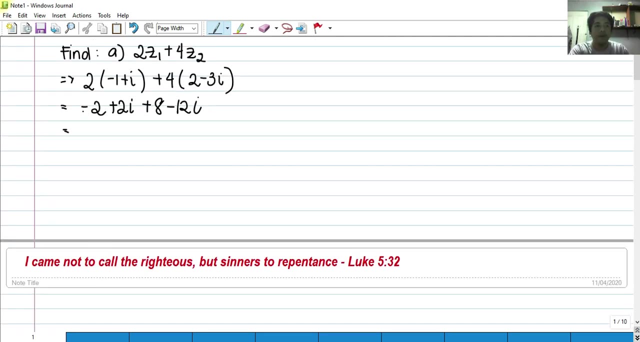 2 times i, that's plus 2i. Then we have plus 4 times 2 is 8.. 4 times negative 3i is negative 12i. So we can simplify some of the values in real part and in the imaginary part. 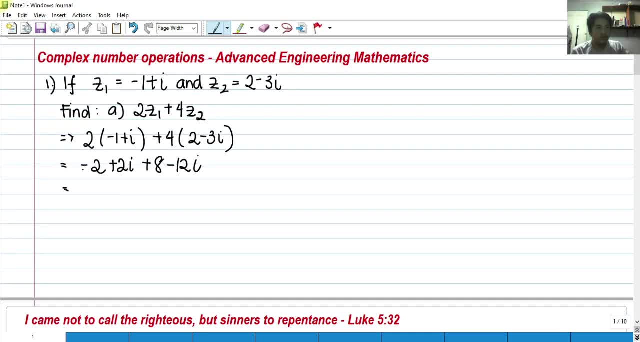 So we are going to simplify. So we can simplify: negative 2 plus 8,, that is obviously 6.. And then we have plus 2i, positive 2i, minus 12i, that is negative 10i. So this is our answer for our first item. 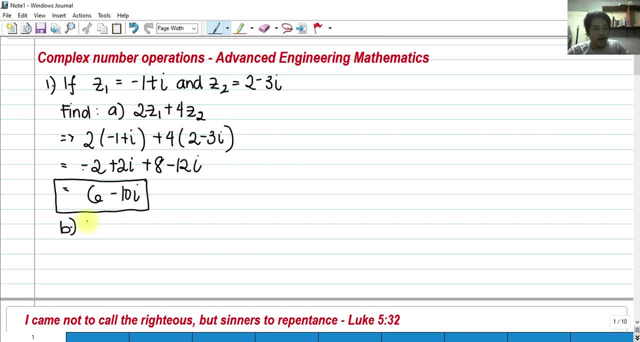 So for letter B we shall be finding z sub 1 multiplied by z sub 2.. So if we do this, of course we have z sub 1, it is negative 1 plus i, then multiplied by z sub 2, which is 2 minus 3i. 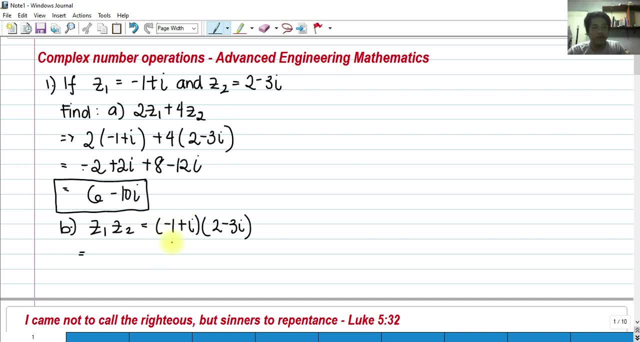 So we will apply FOIL here. So first, negative 1 times 2, that's negative 2.. Outer, we have negative 1 times negative 3i, that's plus 3i In the inner. we have plus 2i in the last. 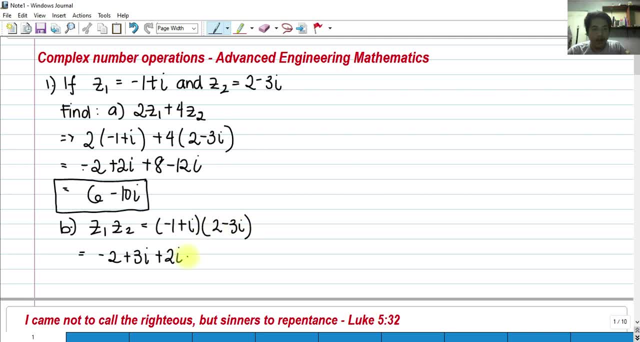 Positive i minus Multiplied by negative 3i, that's negative 3i squared. And if we encounter i squared, take note that because i is equal to square root of negative 1, i squared, therefore, is equal to negative 1.. 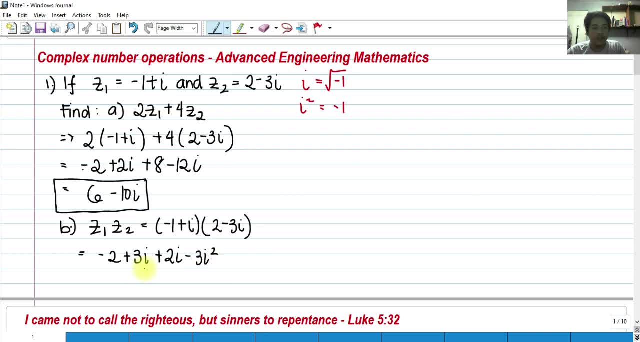 So we can simply reduce this into 3 times negative 1. So we have negative 2 plus 3i plus 2i minus 3 times negative 1. Because i squared again is equal to negative 1. Continuing our operation or our solution: negative 2, okay, and then we can simplify this as positive 3. 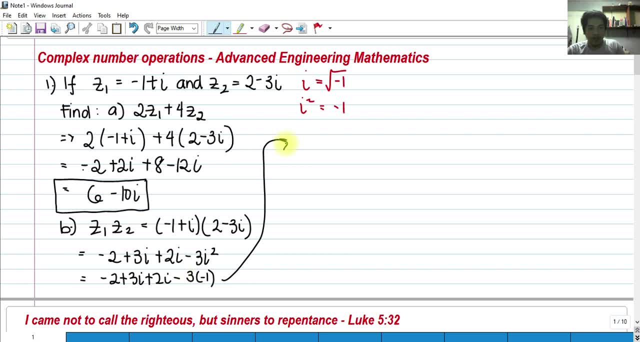 because we have negative 3 times negative 1, that becomes positive 3. So 3 minus 2 would be 1. Then we can add this 2. Then we have plus 5i. So that's how simple it is. on operations of complex. 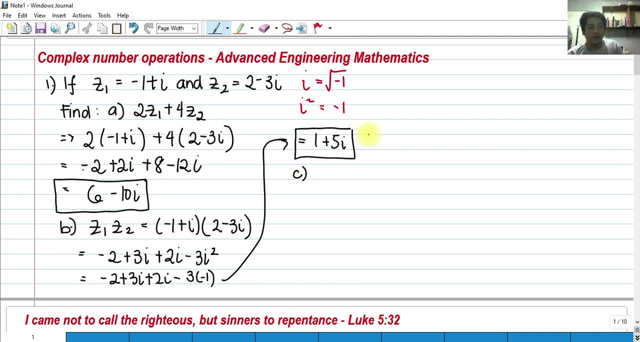 So let's try another one for letter C For our problem. here we have 3z of 1 minus 2z of 2.. So how are we going to do this? 3 times negative 1 plus i minus 2 times z of 2, but that's 2 minus 3i. 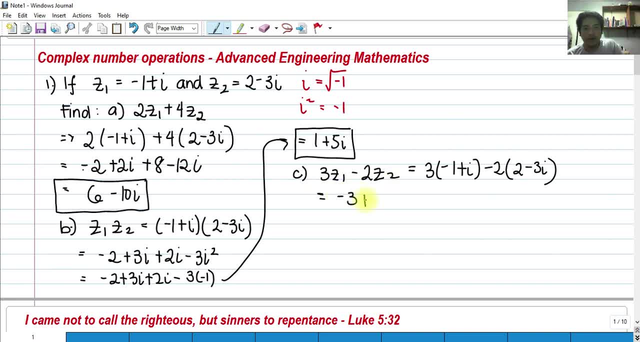 Again, we should distribute this: We have negative 3 plus 3i. Then we have- don't forget to distribute also the minus sign Due to the subtraction. So we have negative 4.. Then we have plus 6i. 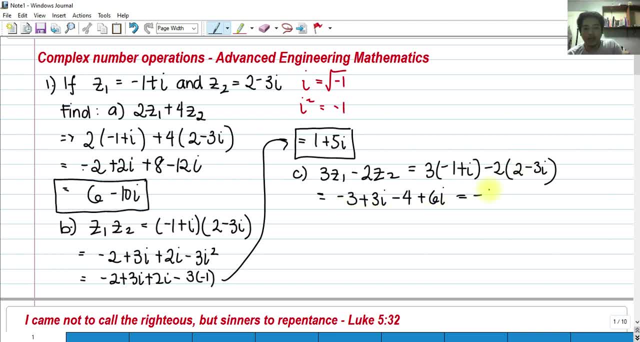 So we can simplify this: Negative 3 minus 4, that's negative 7.. We have 3i plus 6i, that's 9i. So this is our result, The final answer. Okay, for letter D we should try to find z of 1.. 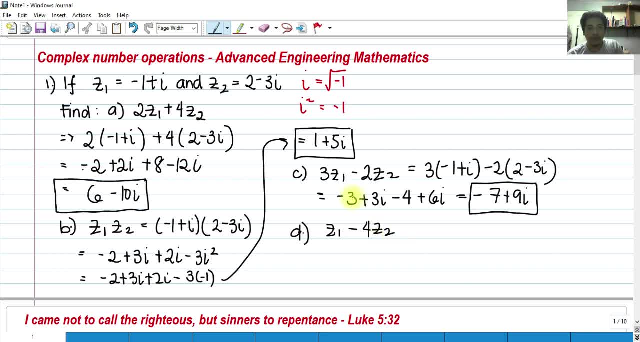 Okay, minus 4 times z of 2.. So we have Negative 1 plus i minus 4 times z of 2, that's 2 minus 3i. Then we have negative 1 plus i, that's negative 8.. 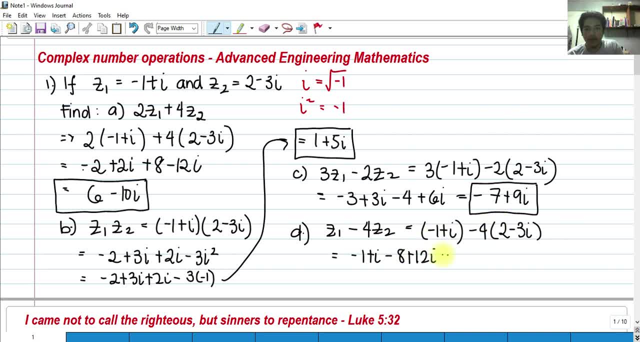 Distribute this negative 4, and then we have plus 12i. Simplifying, we have negative 1 minus 8,, that's negative 9. And then we have i plus 12i, that's 13 positive i. 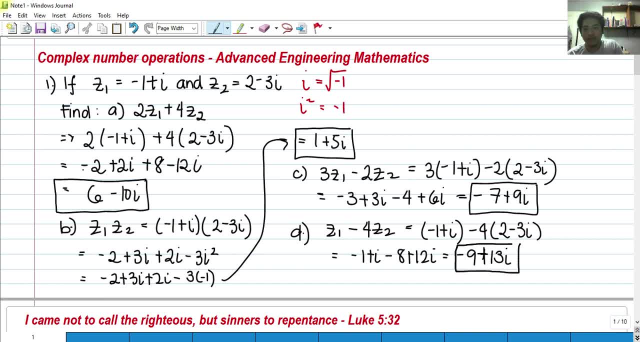 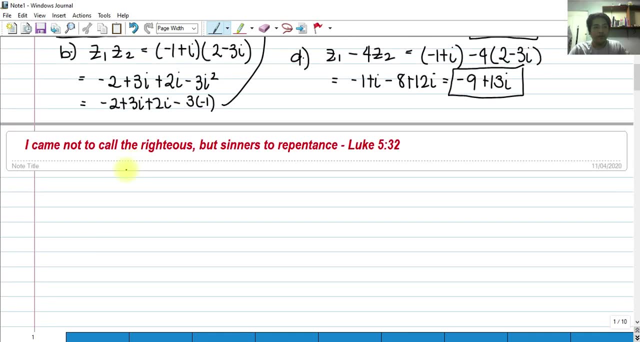 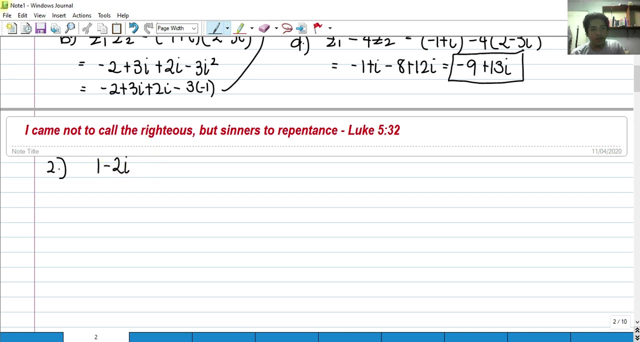 Positive 13i. Okay, Let me just rewrite the plus sign here. Oops, That is our answer. Okay, So for number 2,. okay, that's number 1 only. So how do we find the operation of this complex number? 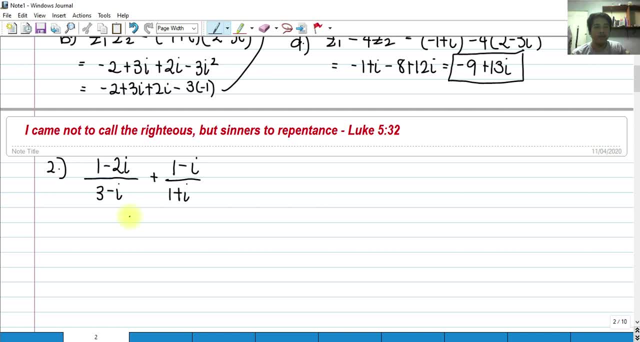 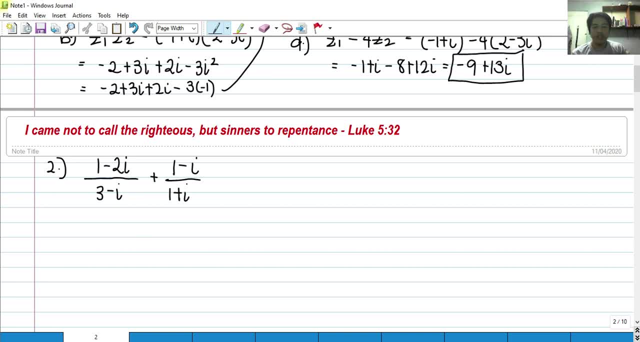 So what are we going to do here? is we, as much as possible, we need to eliminate the denominator containing i. So, in other words, when solving complex problems or complex numbers involving complex numbers, we are going to actually, as much as possible, eliminate the i. 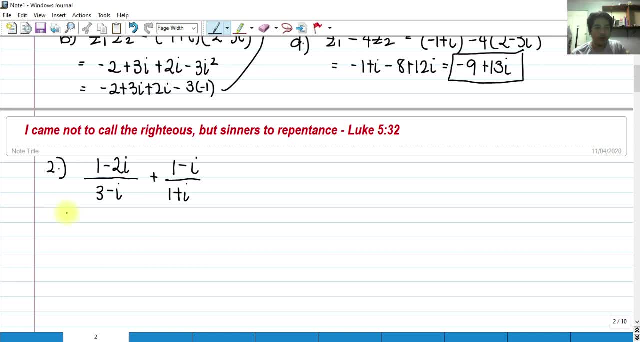 So what are we going to do here is: first, I'm going to multiply each term by the conjugate of each of the denominator. So what are we going to do? again, That is 1 minus 2i, 3 minus i. 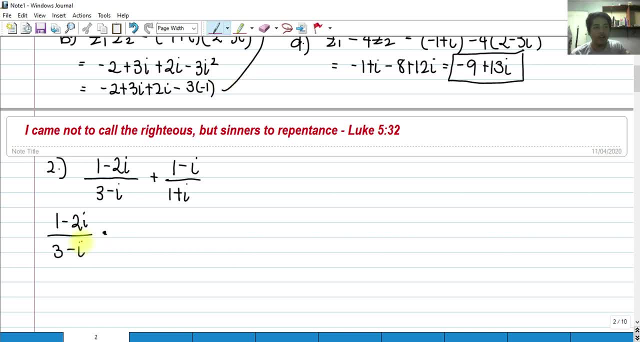 Now I'm going to multiply this, okay, by the conjugate of the denominator. The conjugate of the denominator, we're going to change the sign, okay, of whatever it is, And then, of course, we are going to have, let's say, 3 plus i over 3 plus i. 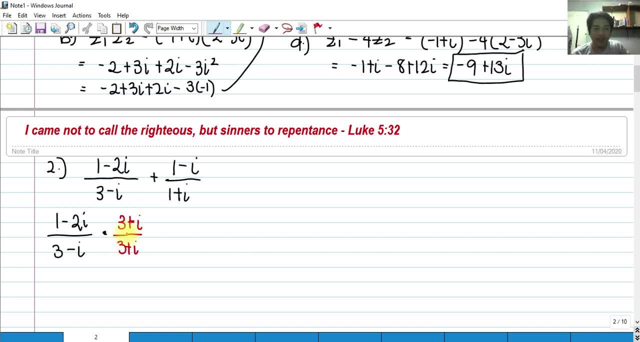 Notice that this is still equal to 1,. okay, We multiply it to this. So still, we are not violating any of the rules here, because we simply multiply it by 1.. But in this way we are going to eliminate the i in the denominator because of i squared. 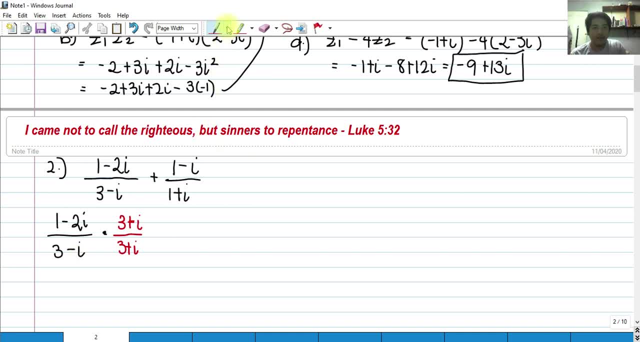 and that is equal to negative 2.. equal to negative: 1.. Of course, if I do that on the first term, I can also do that on the second term, which is 1 plus i. And then, if I'm going to multiply this by the conjugate of the denominator, 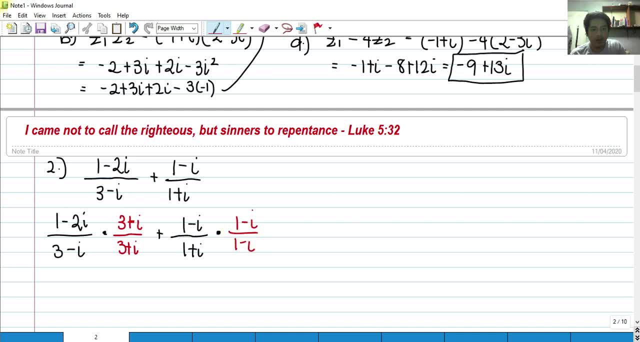 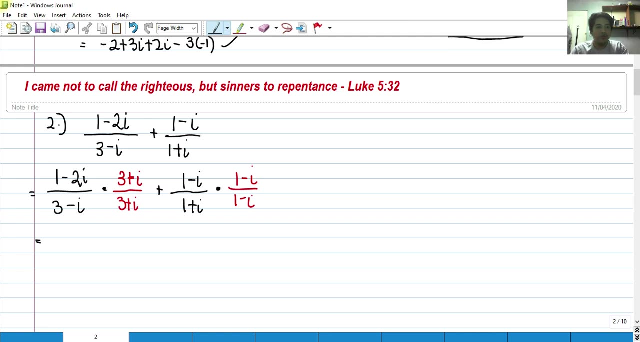 that's 1 minus i, over 1 minus i. So again, we are going to perform our skills here in multiplying complex numbers. So what are we going to do? Denominator times denominator. So we have a denominator. Let me just rewrite this. So we have 1. first, that is 3. Outer, that's 1 times i. 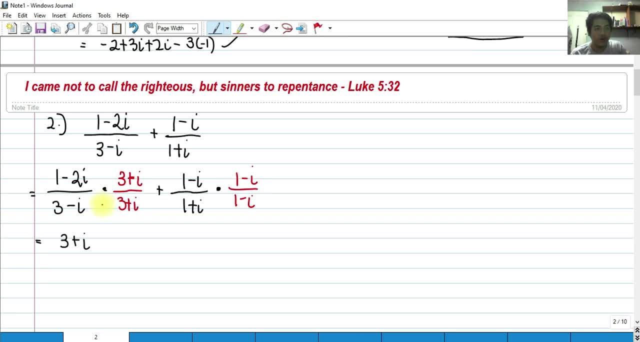 that's plus i Inner we have negative 2i times 3, that is negative 6i, And last we have negative 2i, squared Over. of course, if we are going to really review this, 3 minus i times 3 plus, i remember that we. 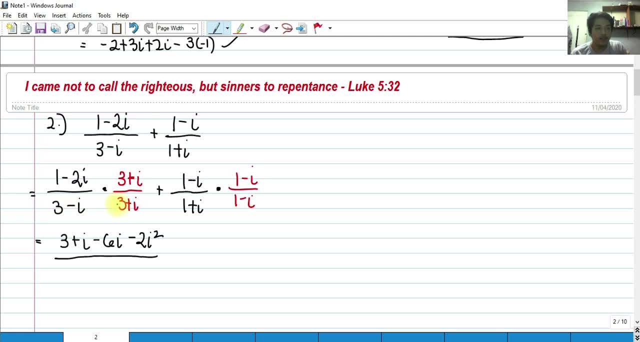 simply multiply this- the first part, first term- and the last term. So that's actually having a x minus y. then we have x plus y in your algebra. So how do we get this? So we are going to have x squared minus. 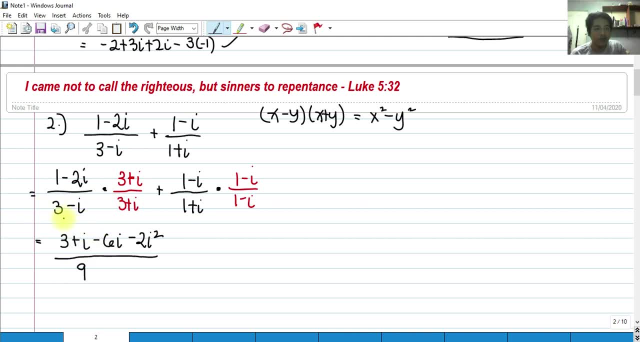 y squared, Of course, the same as this. So we have x squared, which is the 3, then minus i squared. Then moving on to the second term, so we have 1 minus i, We have 1 minus i, both 1 minus i. So 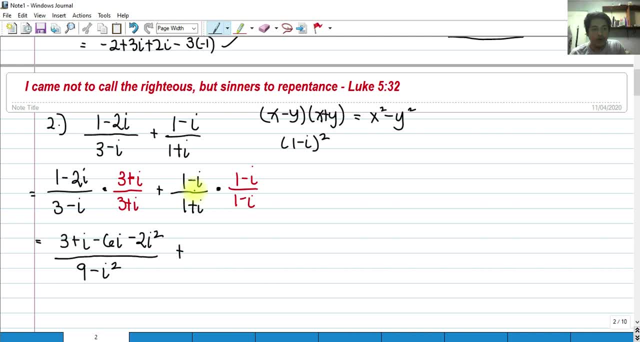 we're going to simply square this So we can have 1 minus 2i. okay, 1 minus 2i plus i squared. If we have 1 minus 2i times 2i, 2 minus 2i squared, it's 1 minus 2i squared, And then we will have 1 minus 2i. 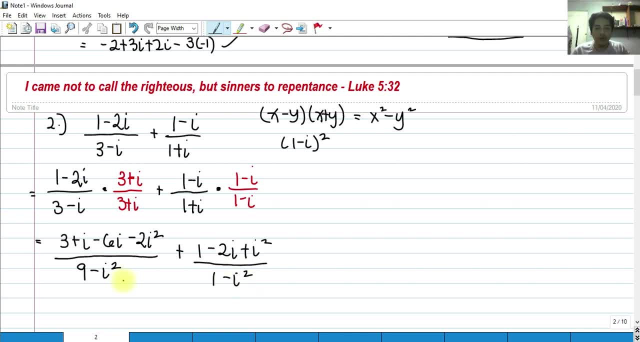 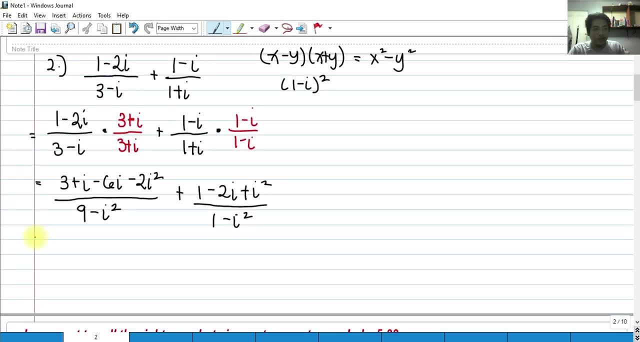 squared. So we have 1 minus 2i plus 1 minus 2i squared. We have 1 minus 2i plus 1 minus 2i squared. So what will happen here is that we simplify first the i. We have plus i minus 6i, that is, minus 5i and negative 2.. 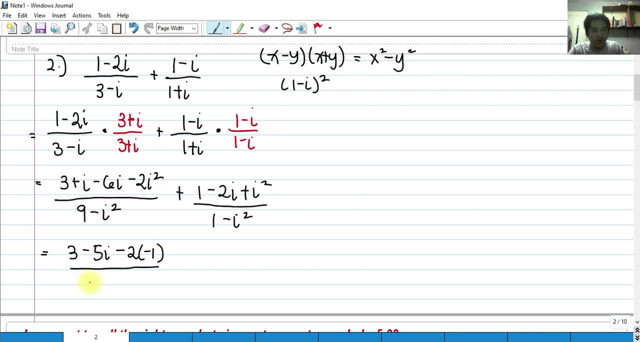 We know that i squared is negative 1 over 9.. We know that this i squared is again negative 1, plus that is 1 minus 2i. We know that that i squared is equal to negative 1 over 1, minus negative 1.. 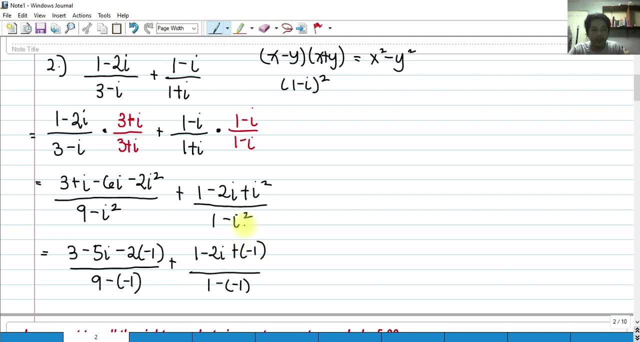 Negative 1,. I'm so sorry. Negative 1, because i squared is equal to negative 1.. So be careful with the sign. So this is minus, but i squared is negative 1.. So we will be having a positive 1.. 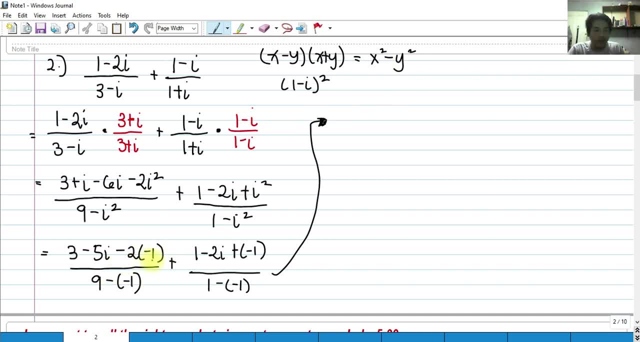 So let's try now. So negative 2 times negative: 1. It will become positive 2. So in that we have 5 minus 5i over 9, minus negative 1. That is over 10. Then we have plus 1 minus 2i. 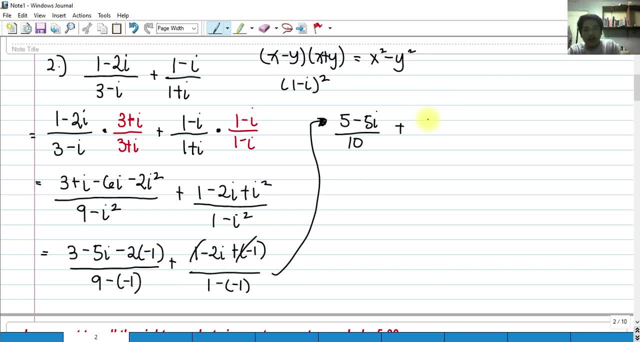 1 minus 1, this would cancel, obviously, So we have negative 2i here. over then 1 minus negative 1, that's 2.. Okay, So what will happen here Here is, this would become 5 minus 5i over 10.. 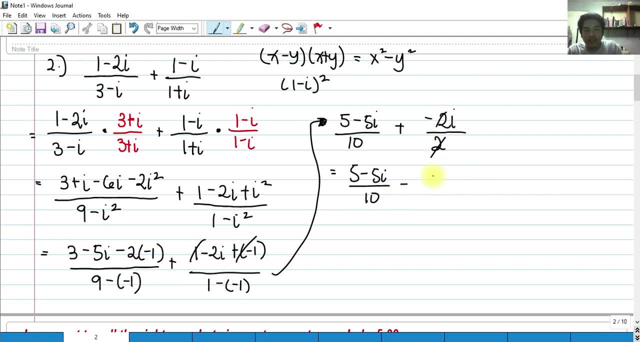 Then we have minus, these 2s will cancel. that will become minus i. But of course we can still factor out 1 fifth here because it's common. Okay, So this can be reduced Or we can- I mean we can- factor out 5.. 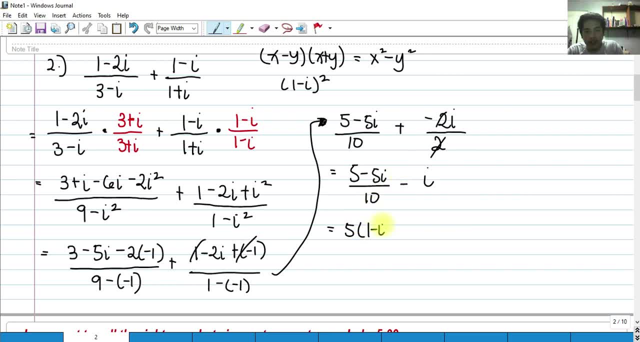 So we have 5. Okay, And then we have 1. 1 minus i. Of course, on the denominator also we can factor 5. That's times 2. 5 times 2 is 10. Minus i. 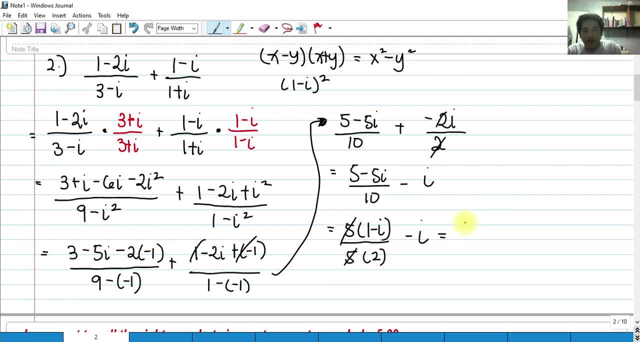 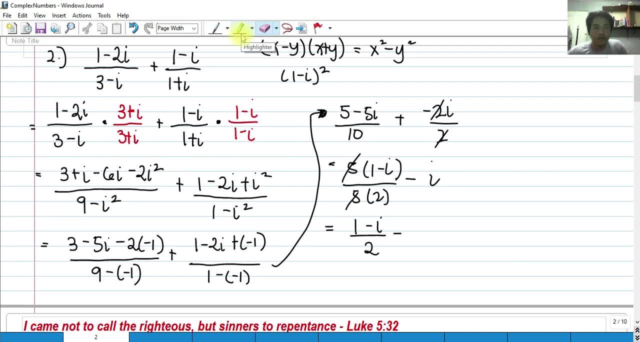 So these 5s will cancel. Then we have 1 minus i over 2 minus i, That is minus i. So if you perform this, okay, we have 1 minus i minus 2i over 2.. Then definitely we have 1, okay, and then minus i minus 2i, negative i minus 2i, that's. 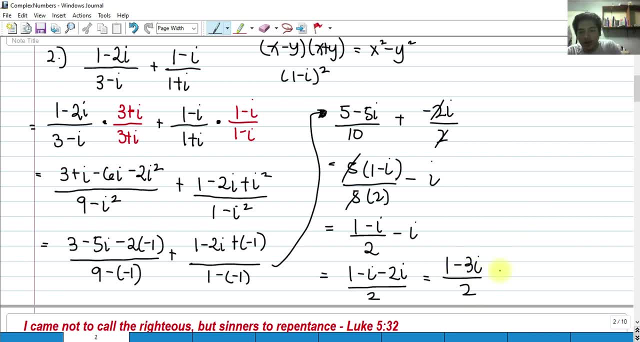 negative 3i over 2.. And of course we can write this as 1 half minus 3 over 2i, And this is our answer for this problem. This shall be our answer. So first, if we have a denominator that is containing i, we should first multiply it. 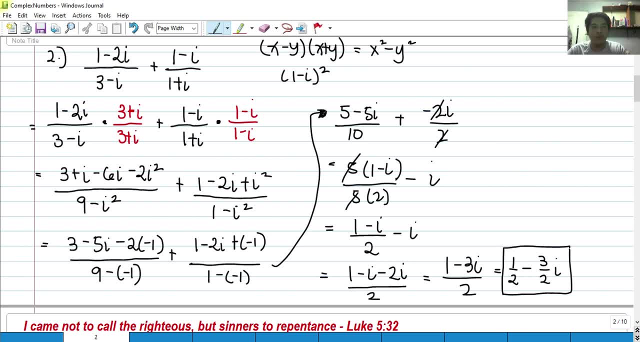 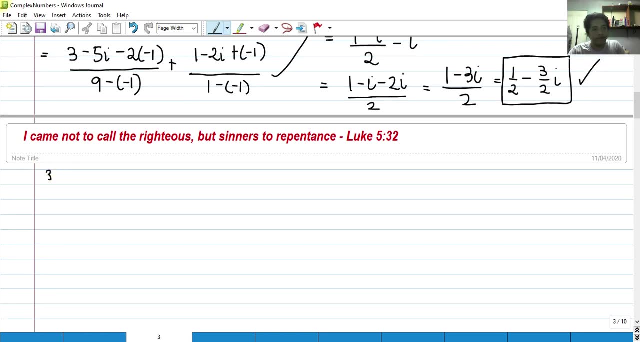 by its conjugate. Okay, In order for us, before we solve the certain operation in the complex number. Okay, So that's the. this is the answer for our problem number 2.. So for our problem number 3, we have 4 plus 5i, quantity: 4 plus 5i multiplied by 4 plus. 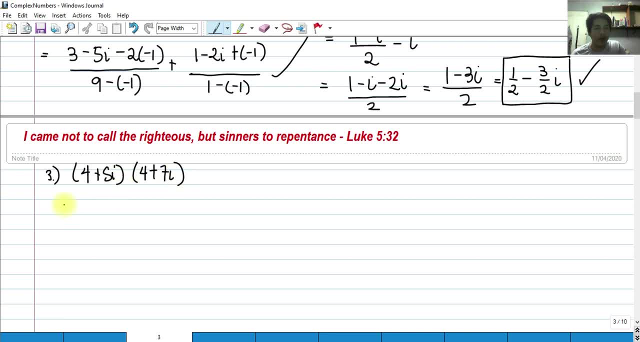 7i. Okay By 4, we have 16 first Outer. we have Okay Plus 28i inner 5i times 4, that's plus 20i. Then we have 5i times 7i, that's plus 35i squared. 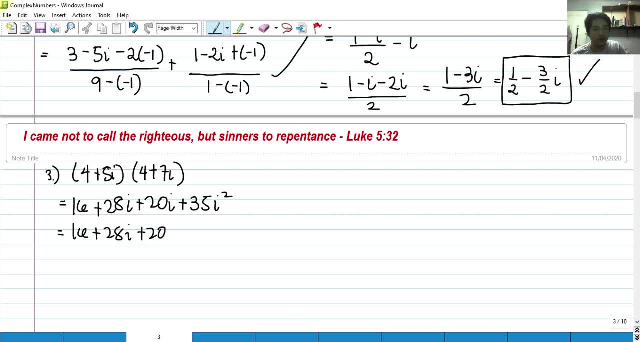 Remember again that i squared is equal to negative 1.. Okay, So we have 16 minus 35 due to negative 1. This 35 is multiplied by negative 1. So that becomes negative 19.. Okay, And then plus 28i, plus 20i, that's plus 48i. 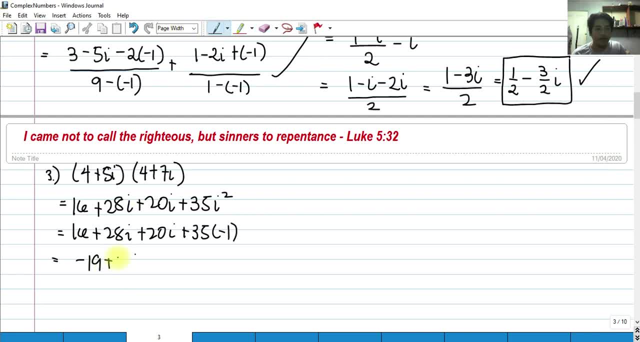 Oops, Let me just rewrite: That's plus 48i. So this is our answer for this problem. It's easy, right? So for number 4, we have 2 squared of 2.. Then we have plus i multiplied by. 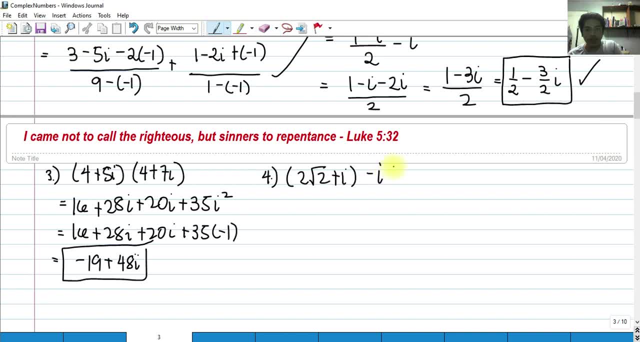 I'm sorry, That's minus minus. i multiplied by 1 plus square root of 2i, Okay. So this is very simple: 2 squared of 2 plus. i Distribute the negative sign Okay And distribute this. multiply it by this term. 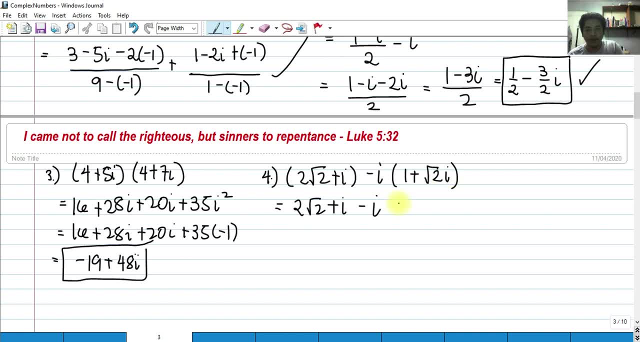 So we have negative i okay, minus square root of 2i squared Okay, And we know that. But if we continue this, that negative i squared is simply equal to negative 1.. So this becomes- this term becomes negative 1 times negative square root of 2.. 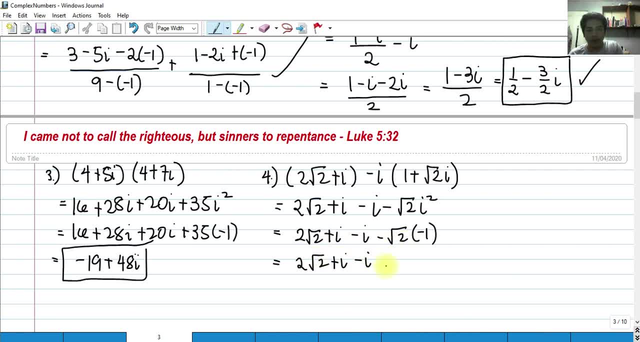 That becomes positive. So we have positive square root of 2.. Plus i, minus- i will cancel, So this is 0. Then we have 2 squared of 2 plus square root of 2. And that is 3 square root of 2.. 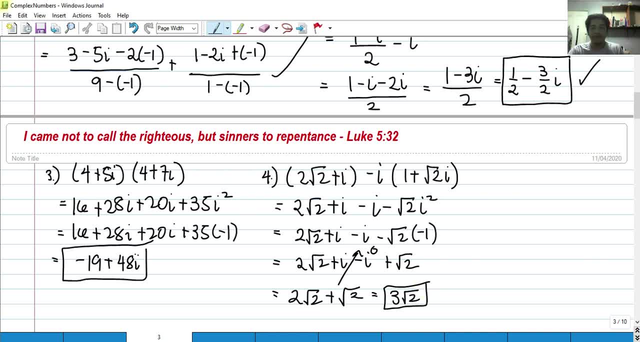 So this is our answer. Okay, For number 5, we have 1 minus i, raised to 3.. So this is also equal to 1 minus i. squared times 1 minus i. Okay, So what will happen is that we're going to square this. 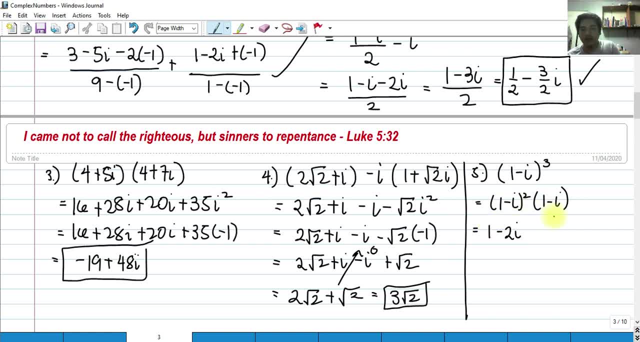 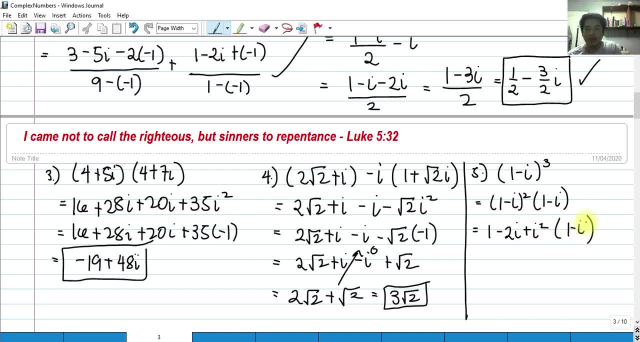 So we can multiply this: 1 minus i Distribute this. So what will happen here? First? first thing to do- I'm sorry- first thing to do is to let this i squared be equal to negative 1.. So we have 1 minus 2i plus i squared. 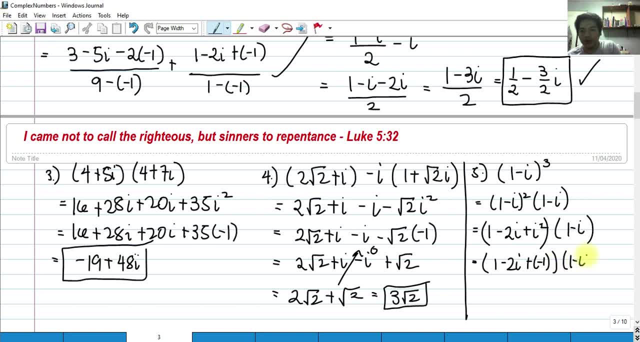 That's plus negative 1. Of course. So, as you can see here, 1 plus negative 1.. Okay, 1 plus. Now 1 minus 1 or 1 minus 1. because of the negative sign here, the 1s will cancel. 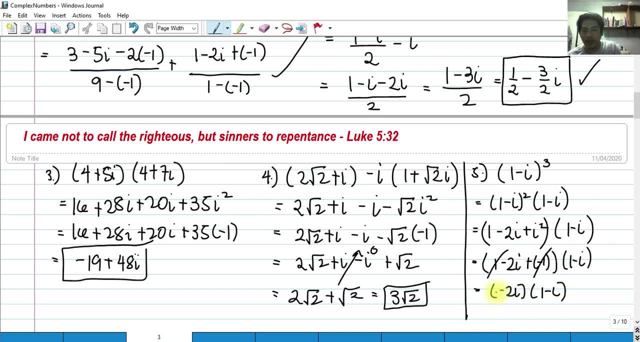 So we have negative 2i multiplied by 1 minus i. So we have negative 2i times 1, negative 2i, Okay, and then negative 2i times negative i. that is plus 2, 2i squared. 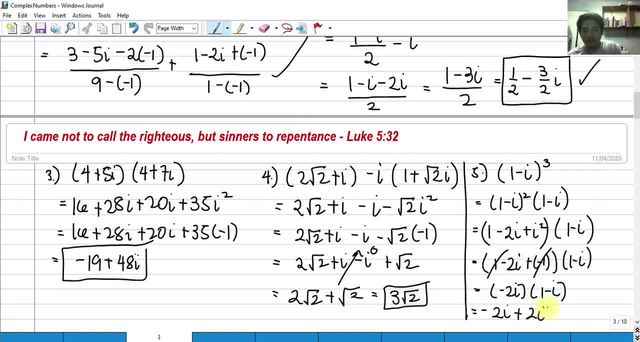 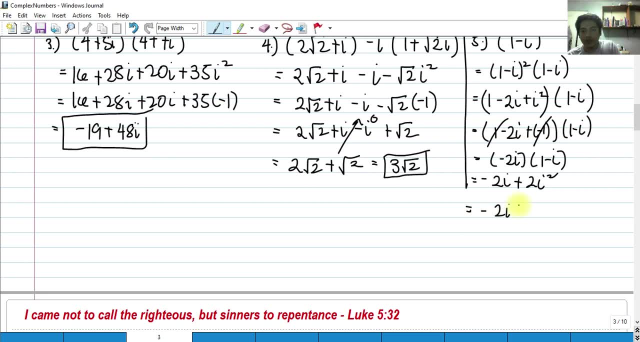 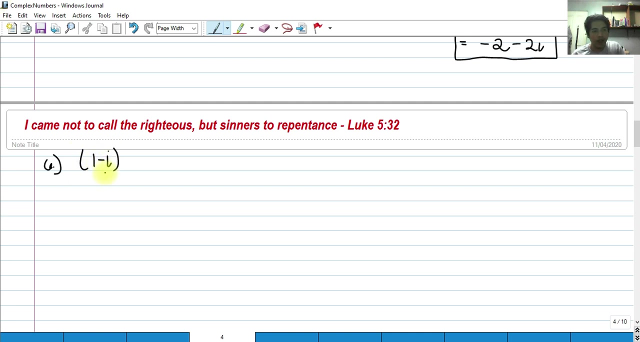 Okay, And our answer- i squared again- is equal to negative 1.. So we have negative 2 minus 2i. So this should be our answer for this problem. Okay, So for number 6, we have 1 minus i over, i minus 1 plus. 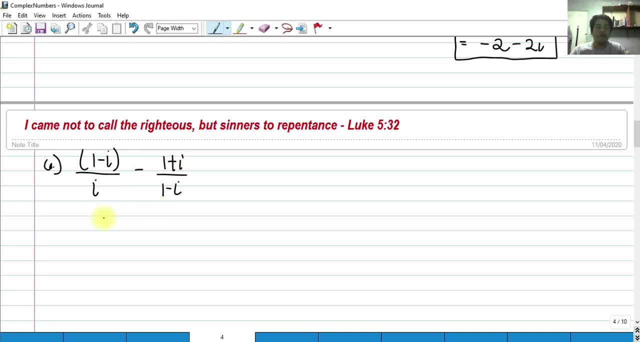 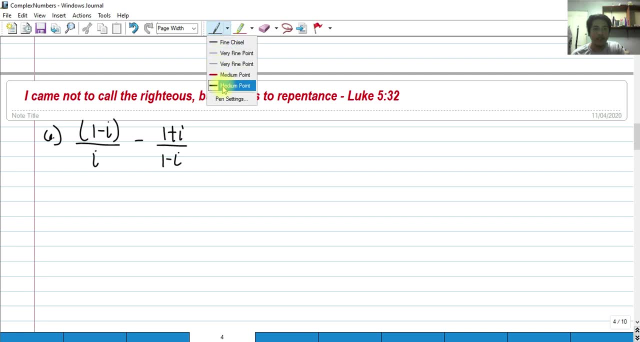 i over 1 minus i. So before we perform the subtraction or subtraction operation, we must again multiply each term by its conjugate. So we have 1 minus i over i. The conjugate of i okay is simply what. 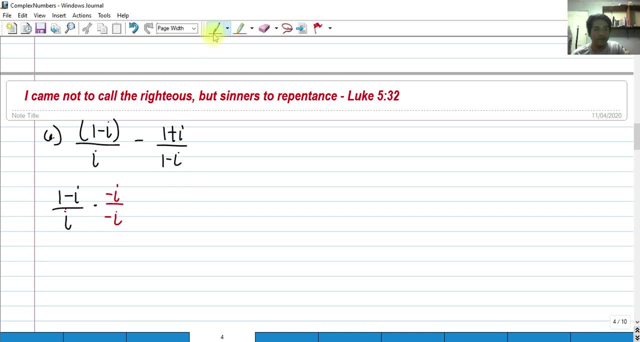 A negative i over negative i, And that is minus 1 plus i over 1.. So 1 minus i. we're going to multiply this by its conjugate. That is 1 plus i over 1 plus i. Okay. 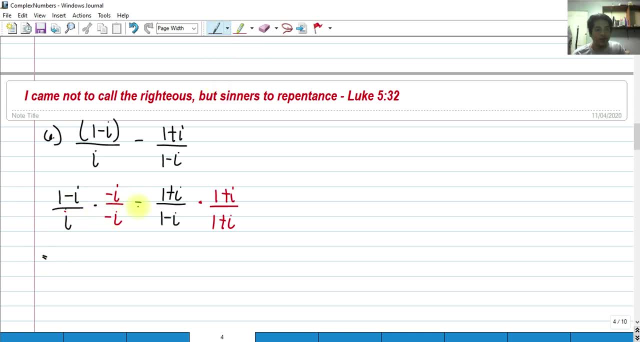 So what will happen here? We have numerator times, numerator That is negative i- Okay, That's plus, i squared over. we have negative i squared here on the denominator Okay, Then we have minus. That is we are going to. 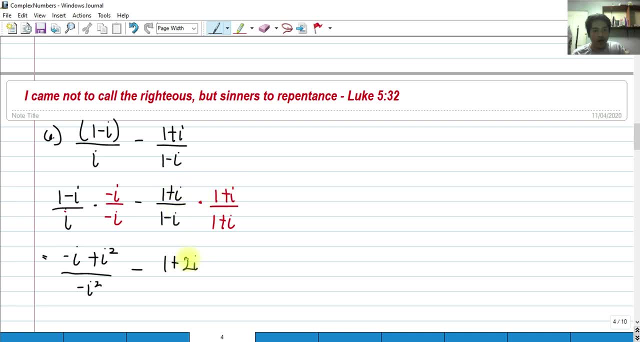 We are going to multiply this, That's 1 plus 2i. Okay Plus, i squared Okay All over 1.. This is again the difference, Okay. So 1 times 1, that's 1.. 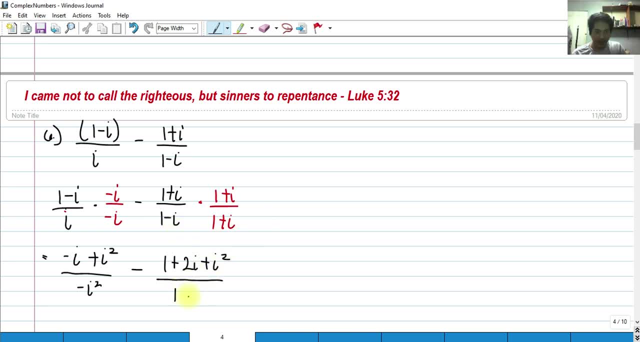 Negative i times positive i. that's negative i squared. Excuse me. So that's negative i squared. So what will happen here Again, replace negative i squared by Negative 1 over negative of negative 1.. Okay, 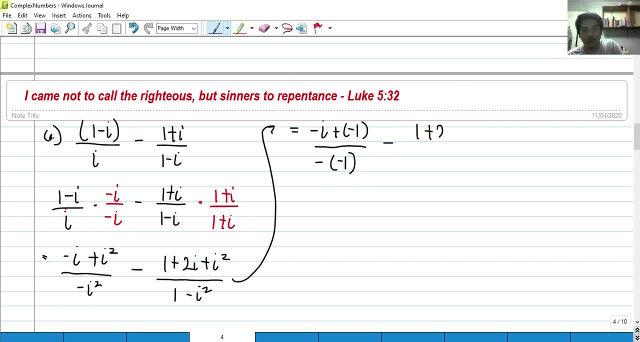 Minus. We have 1 plus 2i plus negative of 1.. Negative 1.. Then we have 1 minus negative multiplied by negative 1.. So we can see here that this is negative 1 minus i over 1.. 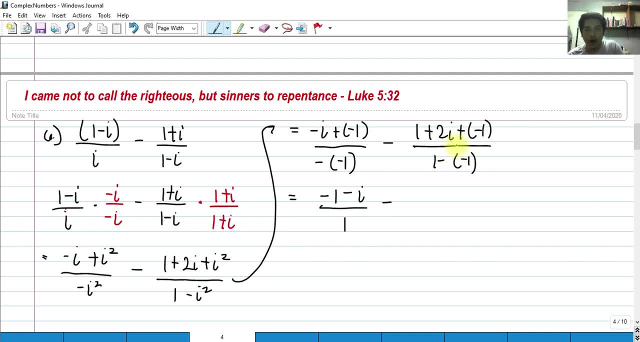 Or simply negative 1 minus i. Then we have 1.. So this 1 will cancel, because 1. Plus negative 1. So this will become 1 minus 1. So this will be canceled. So we have 2i here over 1 minus negative 1.. 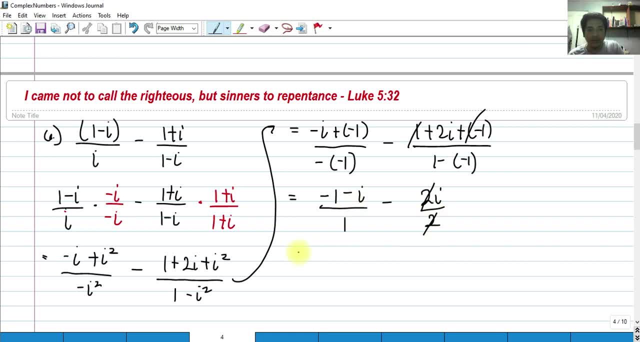 That's 2.. As you can see, these two will cancel, So we have negative 1 minus i, minus i. Okay, That is simply negative 1 minus 2i. So this should be our final answer. So let's go. 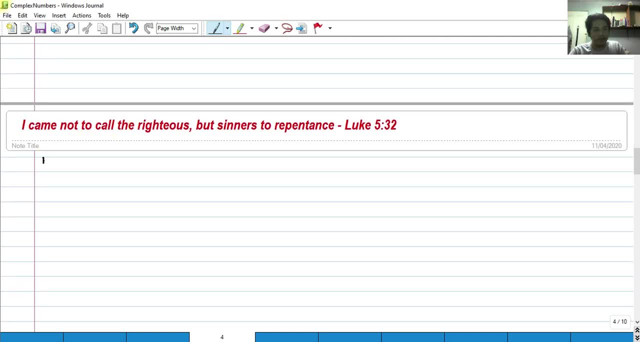 Let's go now for number 7.. If I'm not mistaken, So we have 1 plus i squared over. i So evaluate that It's very easy. So what are we going to do is to again simplify first the numerator. 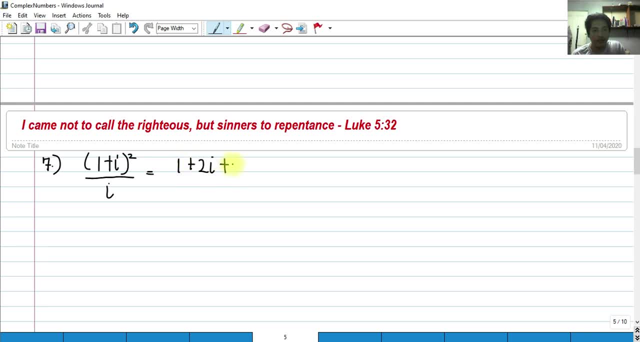 Okay, So what are we going to do? We have 1 plus 2i plus i squared, So we have 1 plus 2i plus i, squared over i. So, as you can see, for this problem, there's no need for you to actually multiply this term into its conjugate. 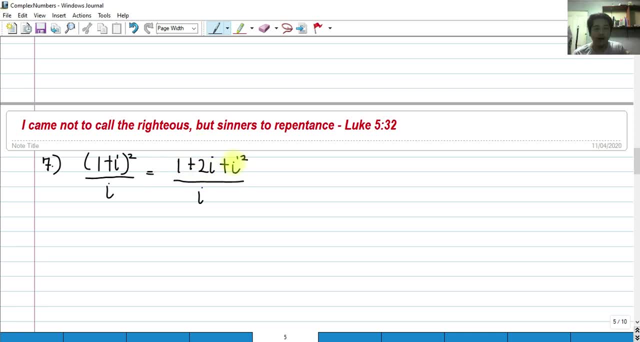 You will see why. Because if you later on simplify the numerator, you see that the i will cancel. So we have 1 plus 2i, Then we have plus i, squared, That's plus negative 1 over i, So this means 1 minus 1.. 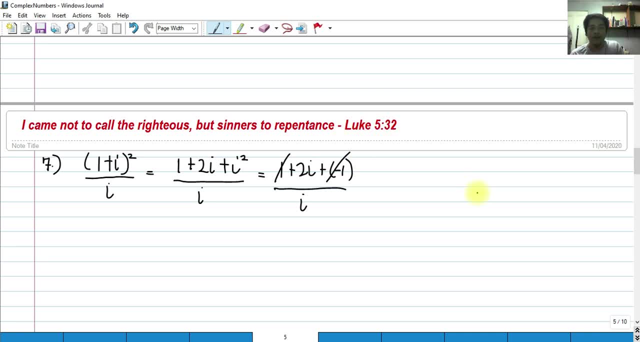 So we have. So we have 1 minus 1.. So we have this. one would cancel Okay. Then we have the remaining 2i over. i The. i will cancel Okay. The. i term The imaginary. 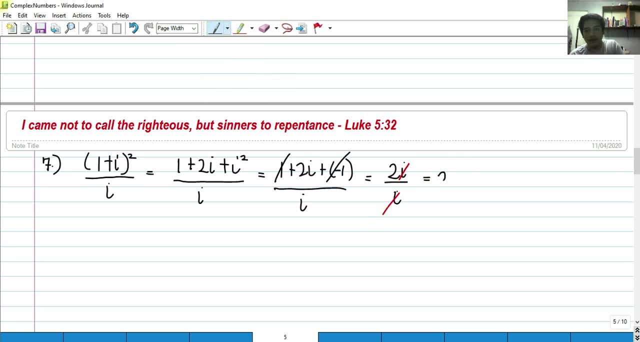 So we have an answer of 2.. Equivalent to 2.. Okay, For number 8, we have quantity squared of 2 minus i Minus i, Quantity 1 minus squared of 2.. So we have 2i. 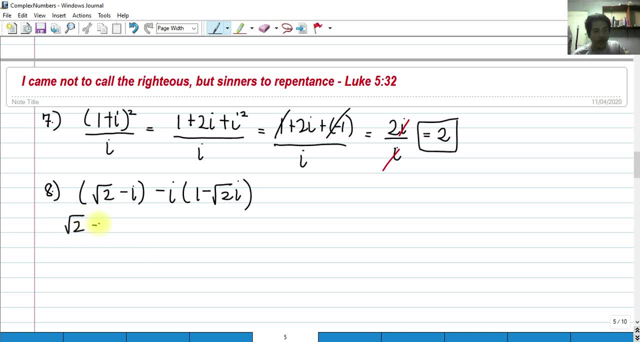 So pretty similar problem we had a while ago. So we can distribute the i together with its sign for this term. So we have negative i. Then we have plus square root of 2i squared. So what will happen here? 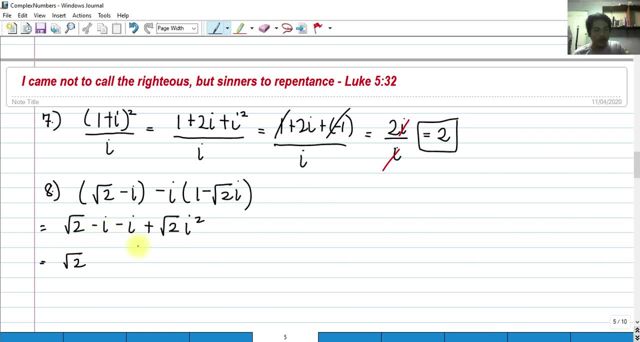 Negative i minus i, We have square root of 2.. Negative i minus i, We have negative 2i And for our i squared that is actually equal to negative 1.. So what will happen? We have square root of 2 minus 2i. 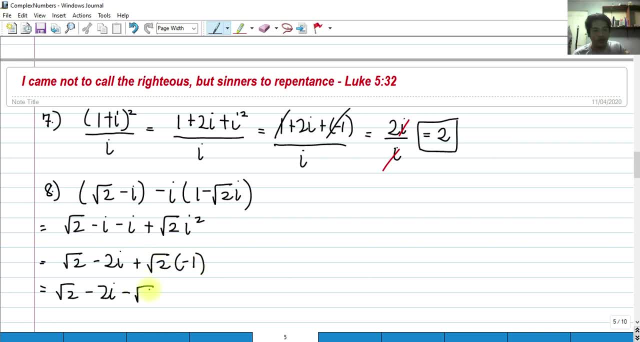 Negative 1 times square root of 2.. Positive square root of that becomes minus square root of 2.. So this 2 will cancel. Then we have an answer of negative 2i. Okay, So for number 9.. 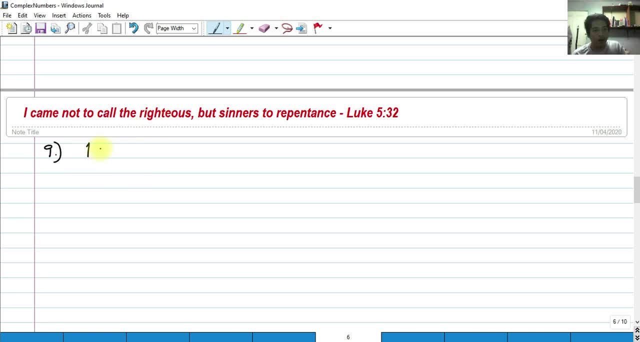 For number 9, we have 1 minus 2i over. Okay, So we have 3 minus 4i, That is plus 2 minus i over 5i. So again, we are going to multiply each term by its conjugate. 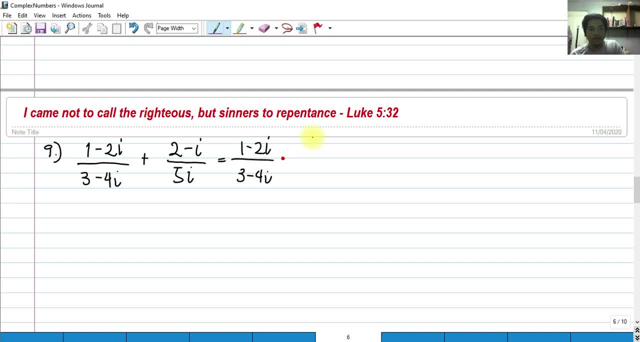 By the conjugate of the denominator. So this must be 3 plus 4i over 3 plus 4i. Then we have the plus. We have 2 minus i over 5i. The conjugate of that is negative 5i. 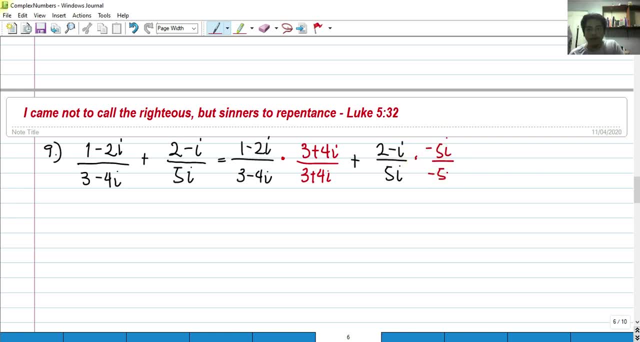 We have negative 5i here, Then we have negative 5i here. Then what are we going to do? Simply perform. Okay, So we have first, 1 times 3.. We have 3.. Outer, we have plus 4i. 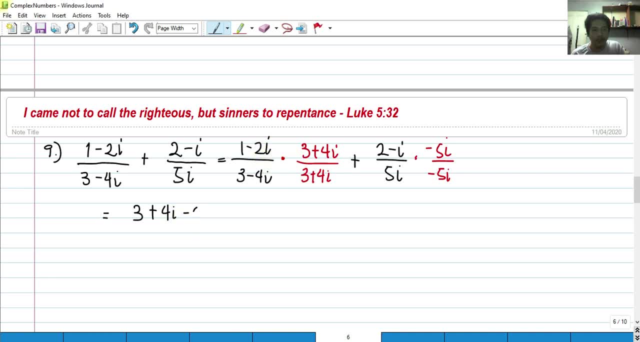 We have inner negative 2i times 3.. That's negative 6i. We have last negative 2i plus 4i. That's negative 6i. That's negative 8i squared over. This is the product of the difference. 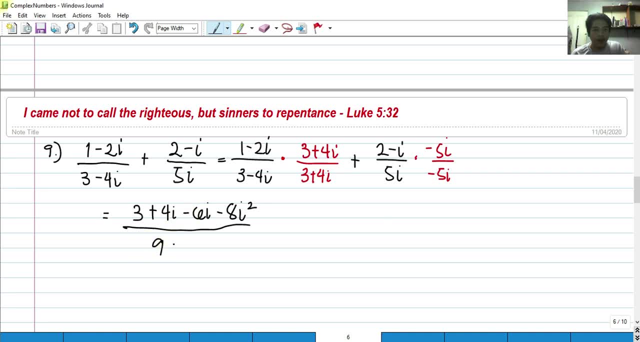 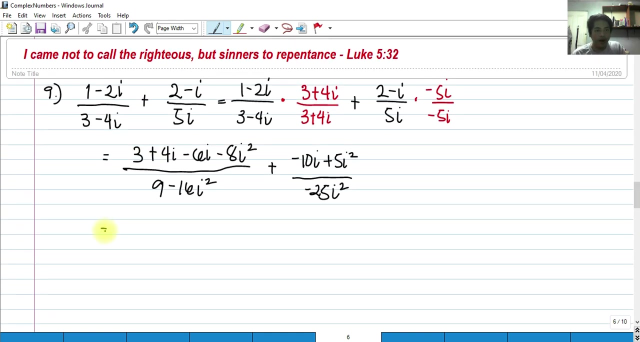 Okay, So we have 9 minus 16i squared, plus of course this. So we have negative 10i, And then we have plus 5i squared over negative 25i squared. So, upon simplifying by substituting i squared, this equals to negative 1.. 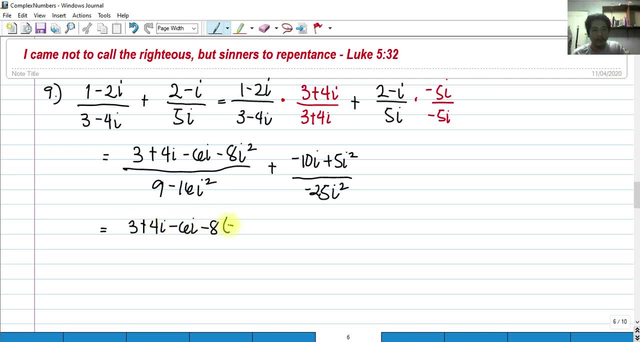 So we have this negative 1 over 9 minus 16.. We have negative 1. Okay, That is plus 5i or 5.. 5 times negative: 1 minus 10i. Okay, Okay, Over negative, 25 times negative 1.. 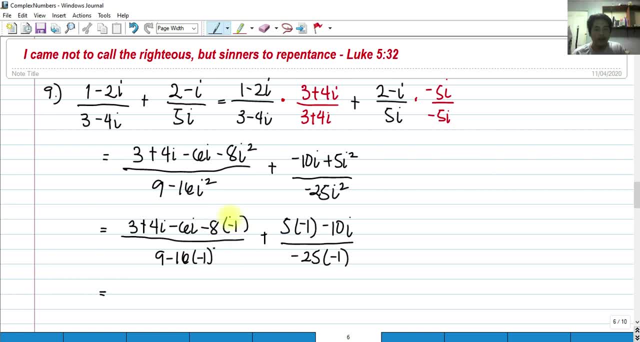 Okay. So let's evaluate So negative 8 times negative: 1. That becomes 8. Okay, Plus 3. That's 11. Okay. Then we have 4i minus 6i, That's negative 2i. 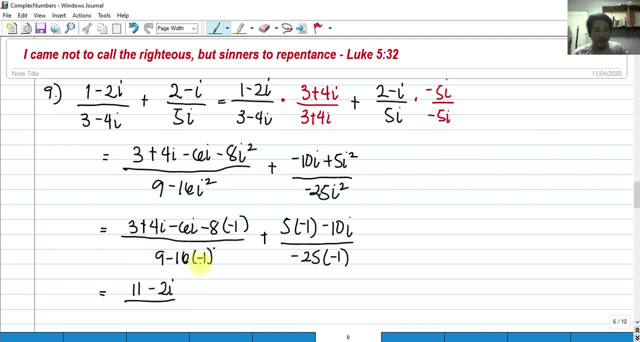 Okay. Then over 9 minus 16 times negative 1. So this becomes plus 16. So 9 plus 16 is over 25. Then we have plus Okay, Then we have negative 5.. 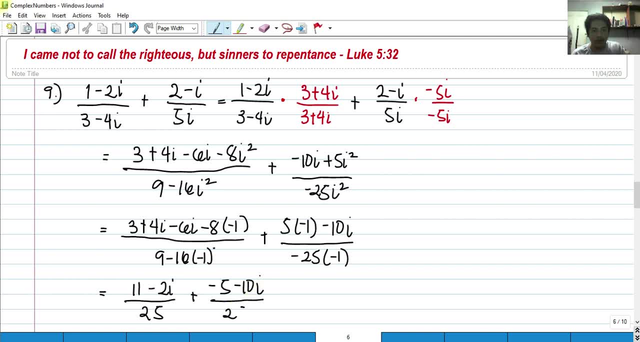 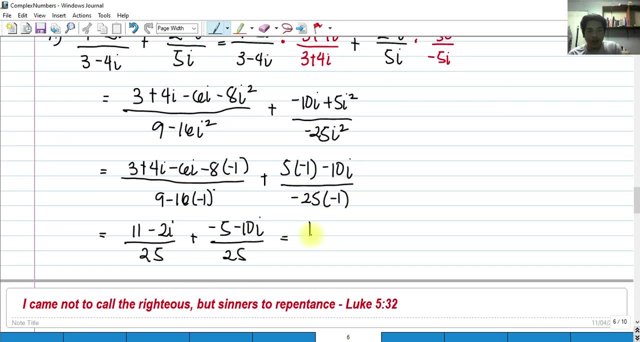 Minus 10i all over 25.. Okay, So, since they have the same denominator, we can rewrite this as 11 minus 2i minus 5 minus 10i all over 25.. And simplify: We have 11 minus 5.. 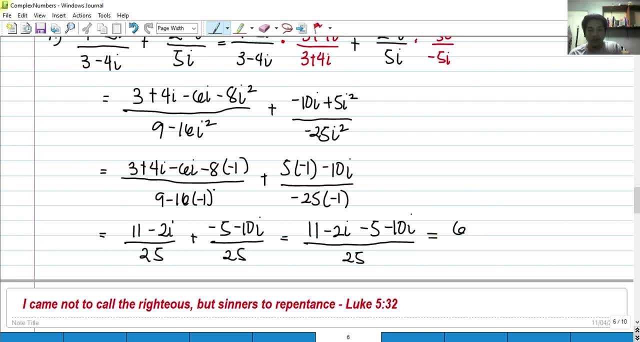 That is 6.. Okay, Negative 2i minus 10i, That's negative 12i. And then we have 6. And then we have over 25.. And that is our answer for this problem, Okay. 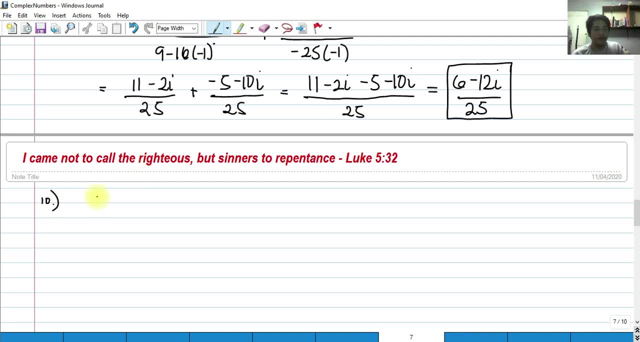 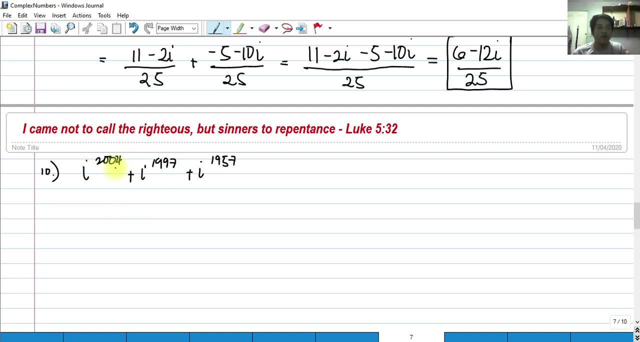 Down to our last problem, For problem number 10.. We're going to solve: i raised to 2004, plus i raised to 1997.. Okay, Plus i raised to 1957 or 1957. So how do we evaluate this? 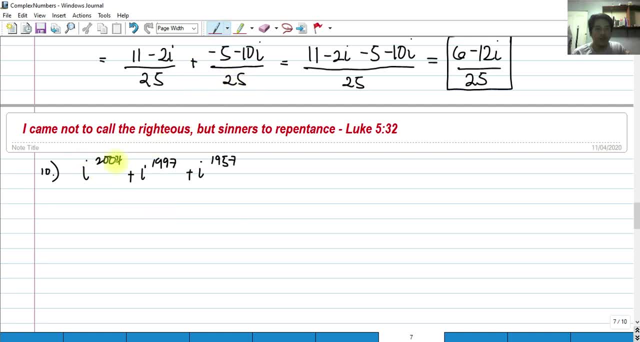 So if we encounter, If we encounter these complex numbers raised to such a huge exponent, so you're going to recall that i is equal to square root of negative 1. We have, i squared is equal to negative 1. i cubed. 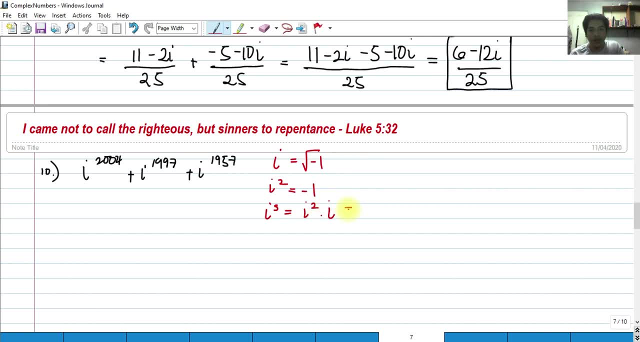 How do we evaluate that? That's equivalent to i squared multiplied by i, But i squared is equal to negative 1.. Then we have times i, Okay, And that is equivalent to negative i, But i squared is equal to negative 1.. 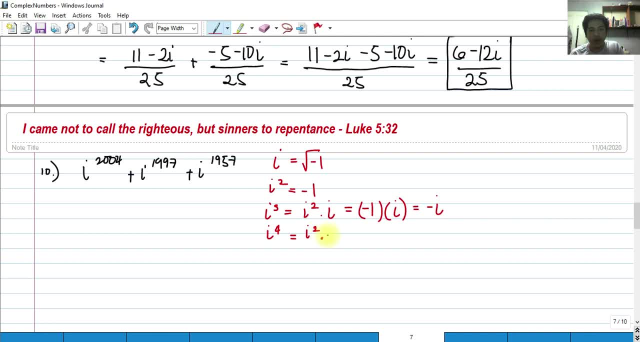 So i raised to 4.. Okay, Remember that it could be split up into i squared times i squared And i squared is simply equal to negative 1. That's times negative, 1. That's equal to 1.. So if we see things such as this: 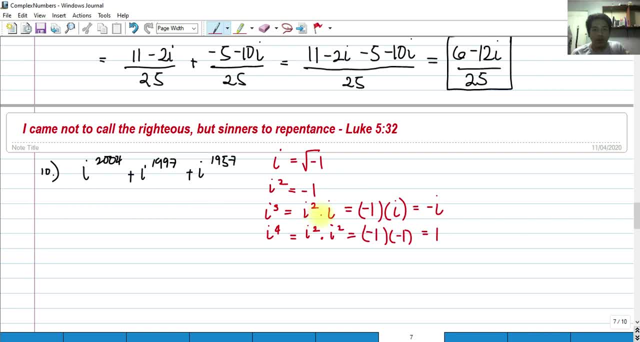 Okay, So we are going to do what we did here in i cubed. So if the exponent is divisible by 4, then automatic that is Equivalent to 1.. Without remainder, if we divide 2004 by 4,. 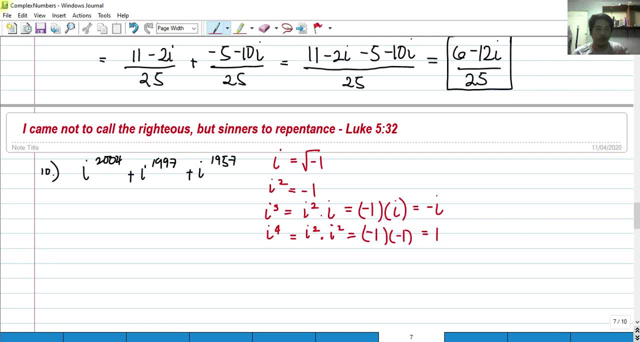 without remainder automatic, that is actually equal to 1.. So 2004, i raised to 2004,. if we are going to divide this by 4, and pretty sure that this is divisible by 4,, that is equivalent to 1.. 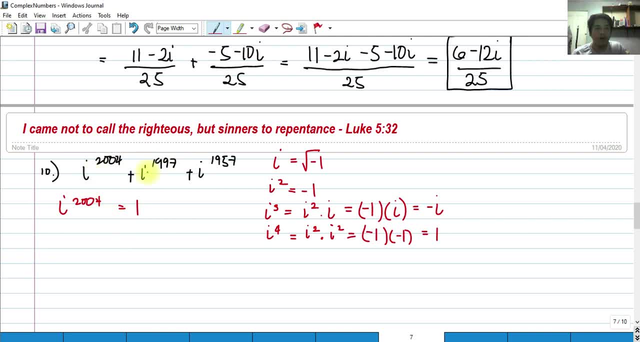 So this term is only equivalent to 1.. How about 1997?? Okay, I don't know, I think. I really think that 1997, i raised to 1, 1,997 is not divisible by 4..